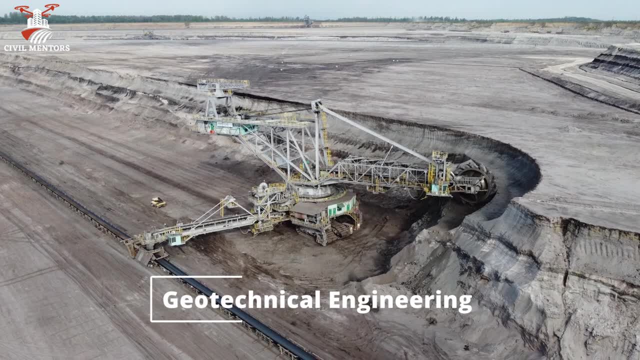 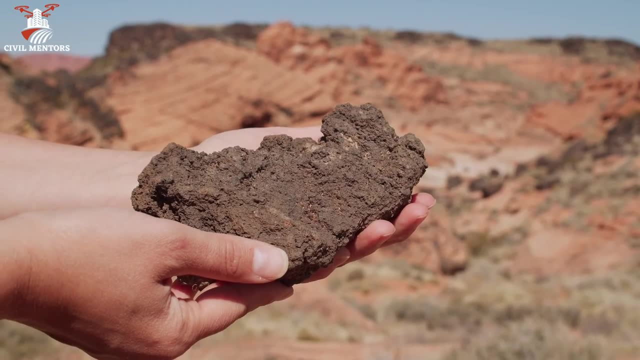 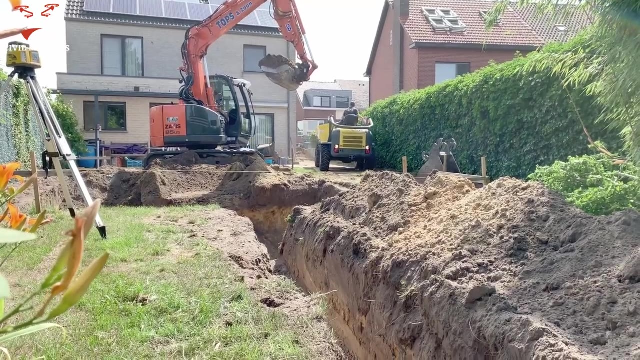 belongings. geotechnical engineering. geotechnical engineers study soil and rock mechanics to determine the properties of these materials and their impact on infrastructure projects, such as the stability of slopes, foundations and tunnels. this knowledge helps them design safe and effective foundations and retaining structures for their construction projects. 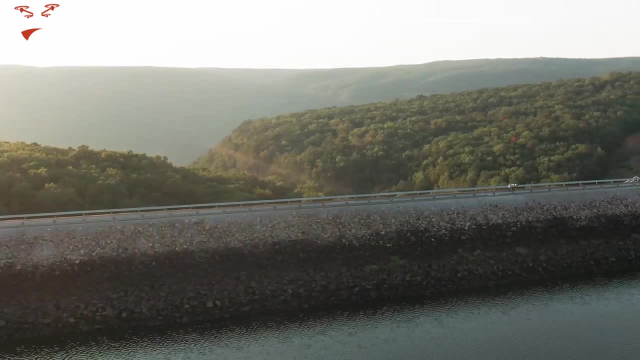 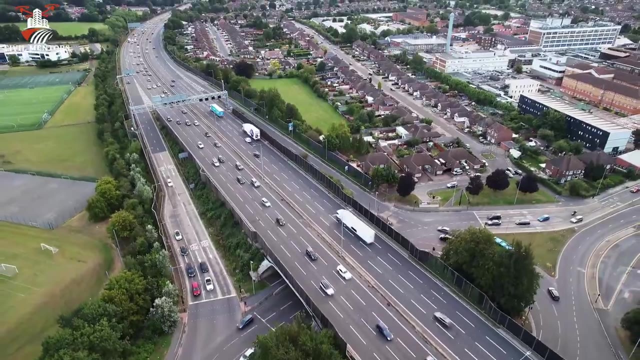 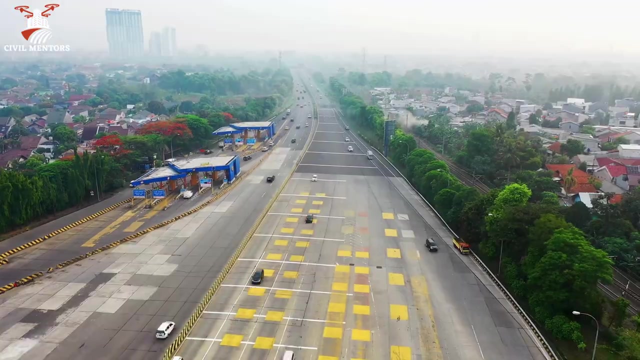 the civil engineering department is responsible for the development of a system of infrastructure structures that can support the weight of buildings, bridges and other infrastructure. transportation engineering: this field deals with the planning, design and operation of transportation systems, including highways, railways and airports, to provide efficient and safe movement of people. 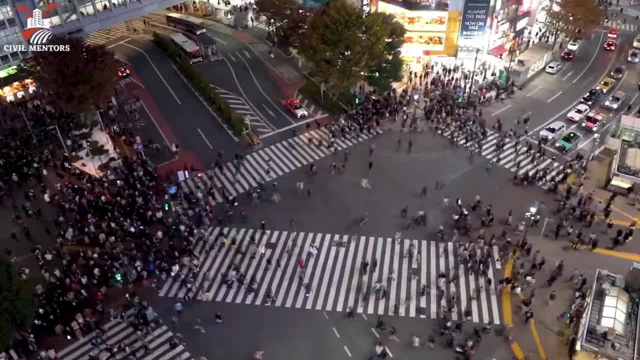 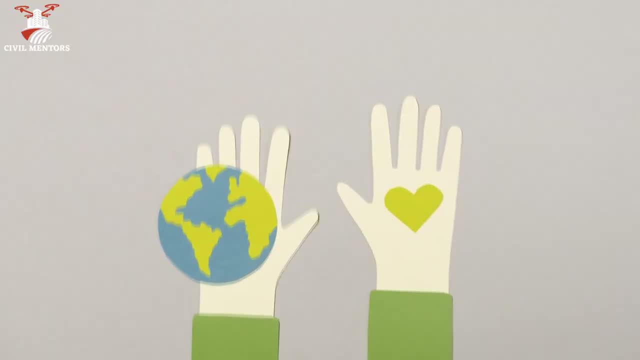 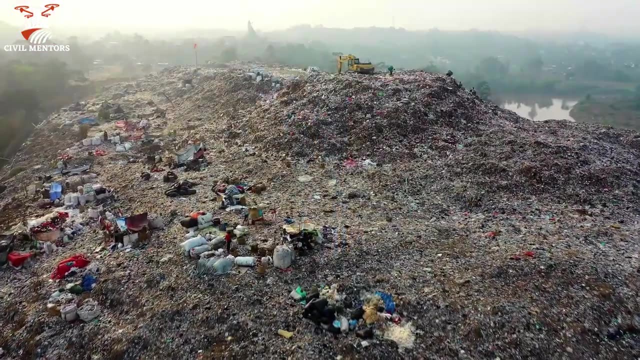 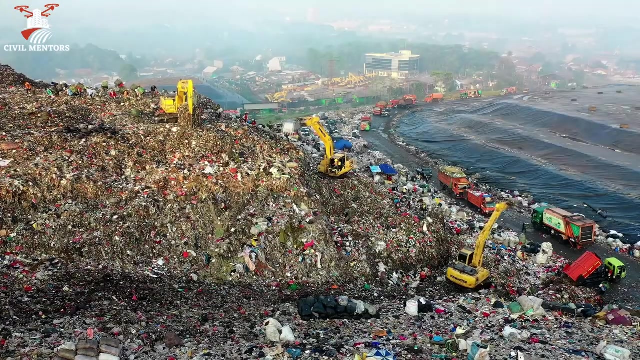 and goods. transportation engineers must consider factors like traffic flow, vehicle dynamics and the needs of pedestrians and cyclists to create effective transportation networks. environmental engineers focus on protecting the environment and public health by addressing issues such as water and air pollution, waste management and sustainable development. they design systems for water and wastewater treatment, air pollution control and solid 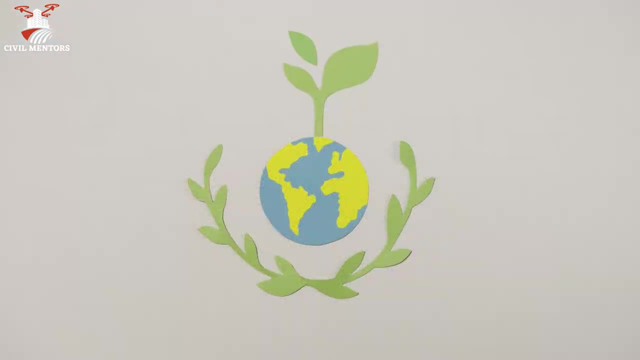 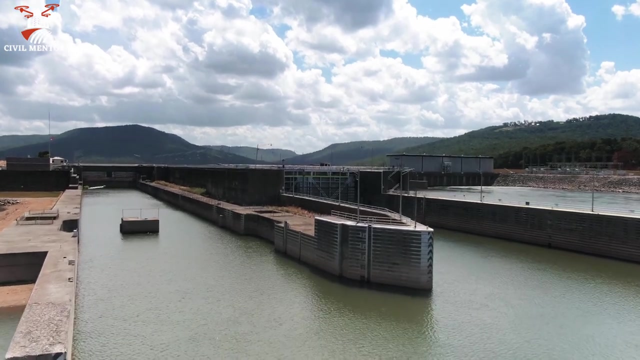 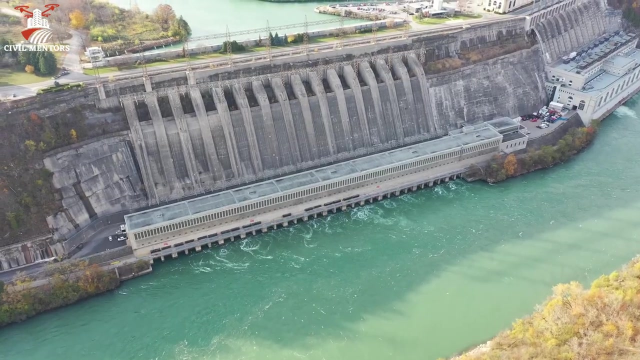 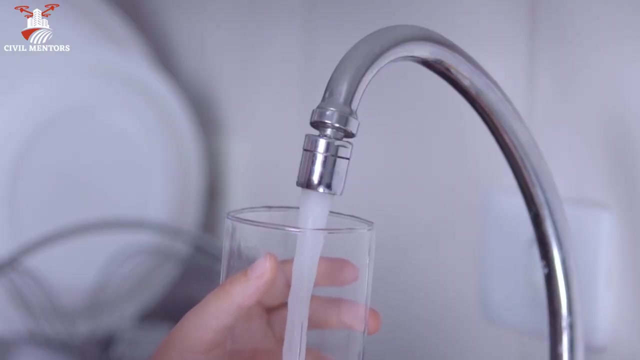 waste management to help reduce the environmental impact of human activities. water resources engineering: this discipline is concerned with the management and distribution of water resources, including the design of dams, flood control systems and water treatment facilities. water resources engineers play a crucial role in ensuring that communities have access to clean and safe water and that water is used efficiently: construction engineering and. 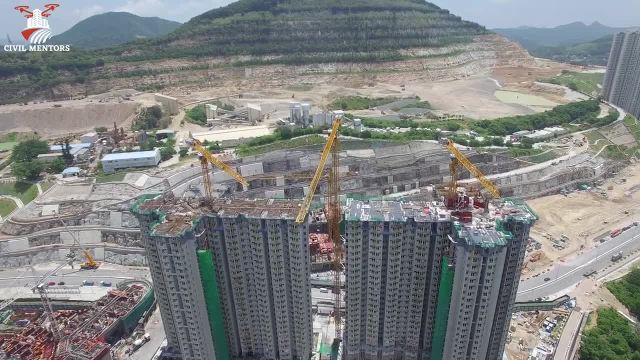 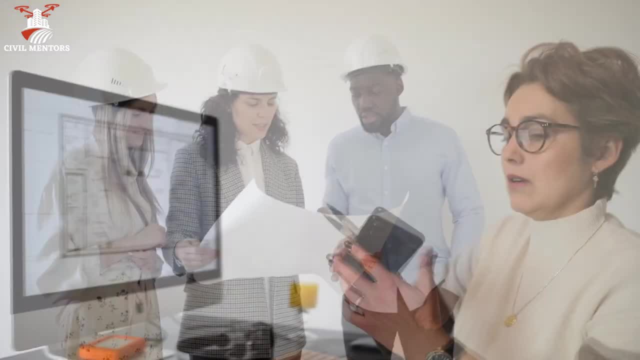 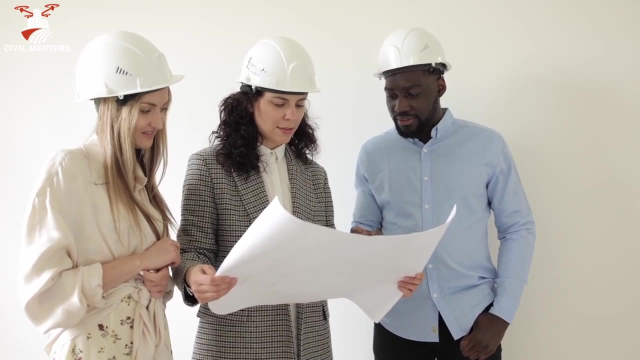 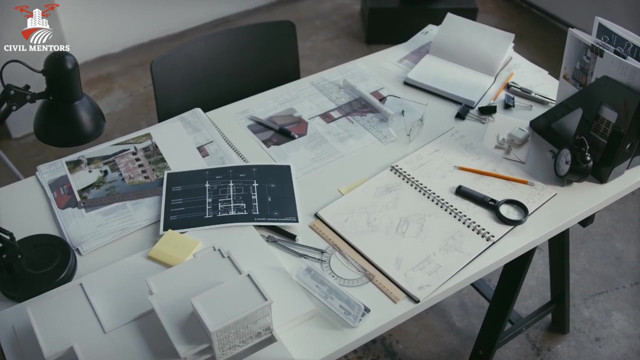 management. this sub-discipline focuses on the construction process itself, including project planning, scheduling, cost estimation and quality control. construction engineers and managers work to ensure that projects are completed on time, within budget and to the required quality standards. section 4: the design process. a critical aspect of civil engineering is the design process. 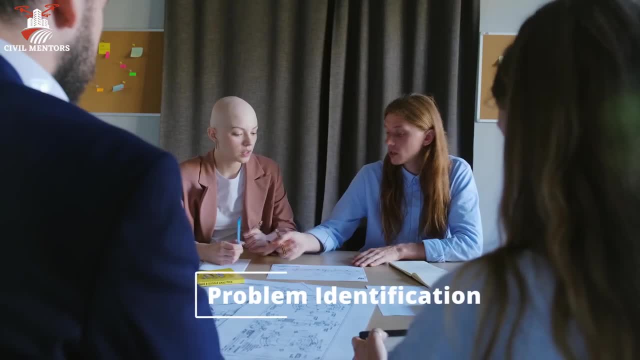 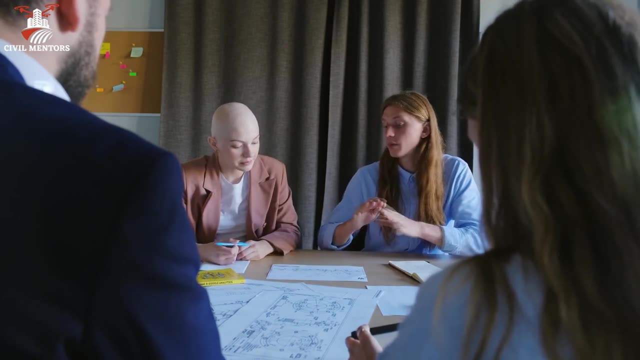 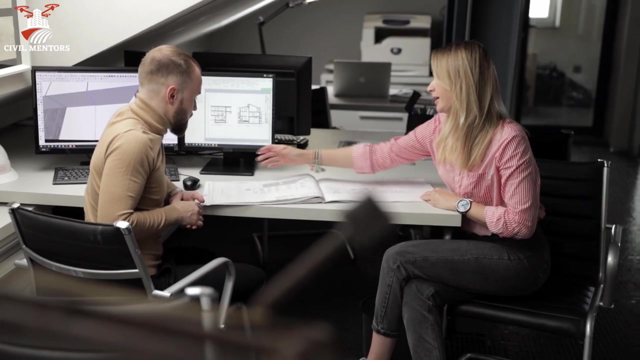 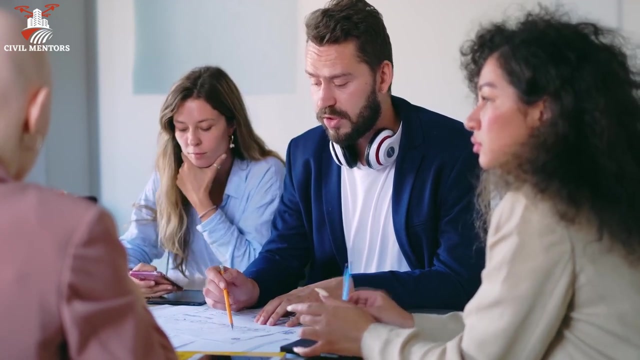 it typically involves the following steps: problem identification: clearly define the problem and its scope, including the needs, constraints and objectives of the project. data collection: gather information about the site, materials, regulations and any other relevant factors. this may involve conducting site visits, consulting with experts or reviewing existing data and studies. analysis: analyze the data and develop mathematical models to determine the. 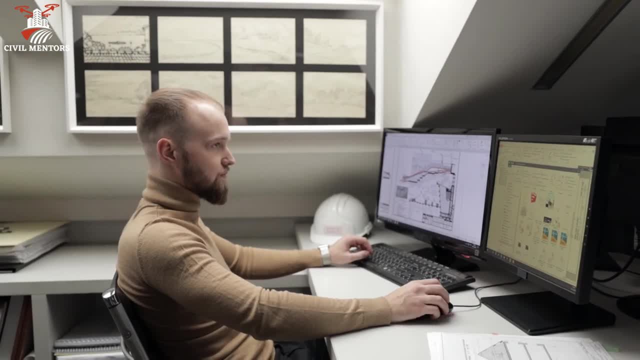 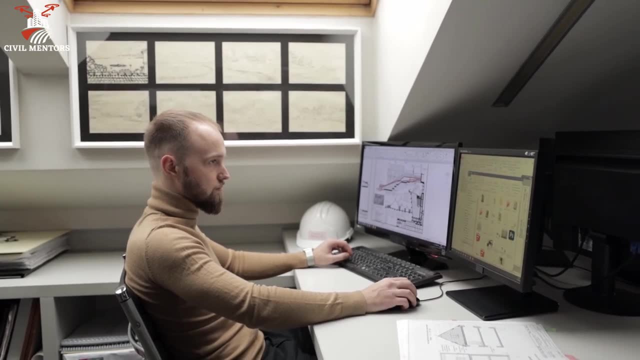 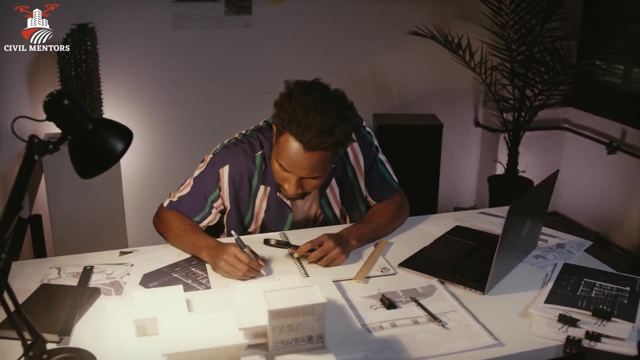 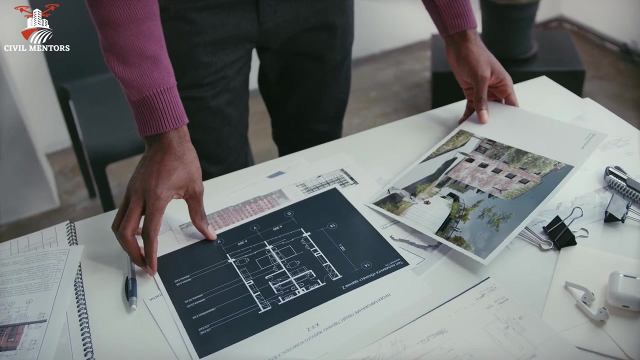 most effective design solution. this may involve using computer simulations, conducting experiments or applying analytical techniques to evaluate various design alternatives. design: create detailed design plans, specifications and drawings that meet the project's objectives and comply with relevant regulations. this step requires the engineer to make informed decisions based on their analysis and knowledge of materials, construction methods and engineering. 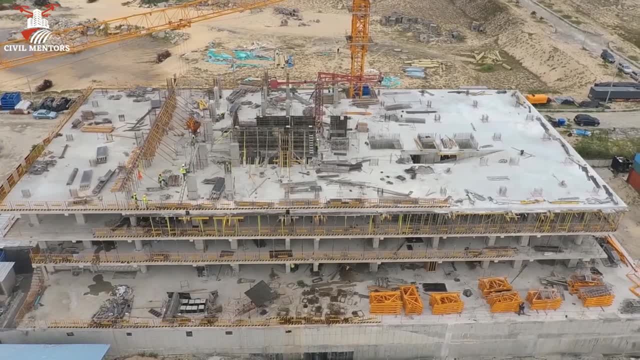 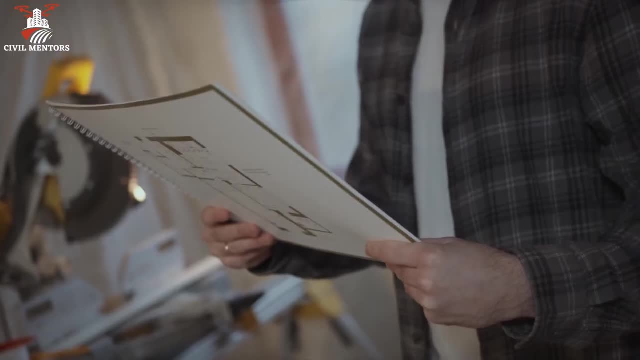 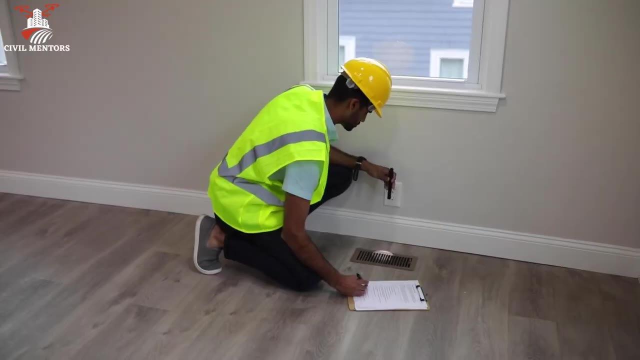 principles construction: oversee the construction process to ensure the project is built according to the design and meets quality standards. civil engineers collaborate with contractors, architects and other professionals to address any issues that may arise during construction. maintenance, monitor and maintain the infrastructure to ensure its continued functionality and safety. this may 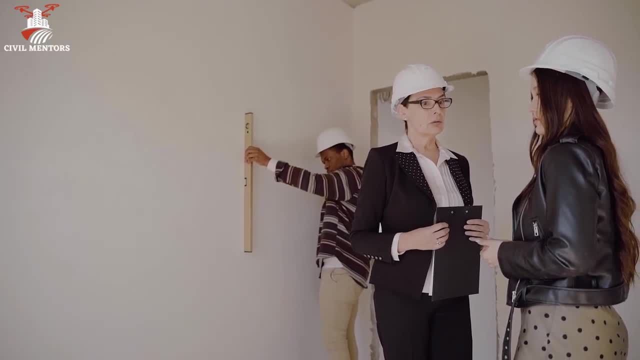 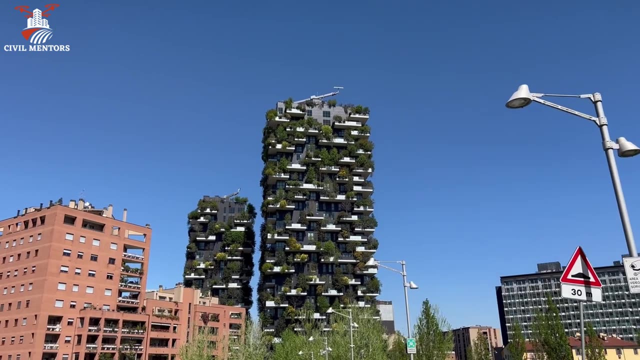 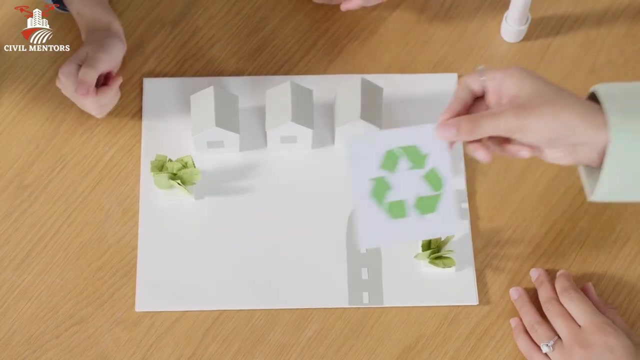 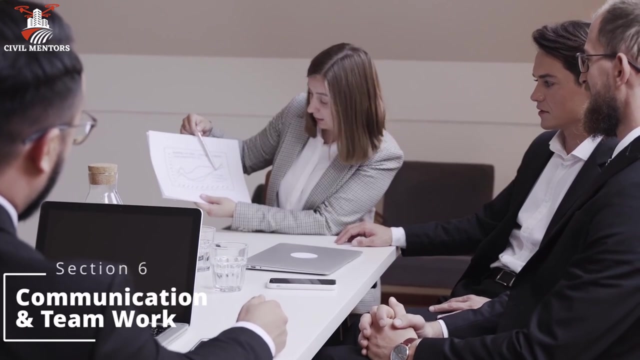 involve conducting inspections, performing repairs or making recommendations for improvements or upgrades. section 5: sustainable and green engineering. sustainability is a vital consideration in modern civil engineering. engineers must develop infrastructure projects that minimize environmental impact, reduce resource consumption and promote social well-being. section 6: communication and teamwork. effective communication and teamwork are essential skills for civil engineers. 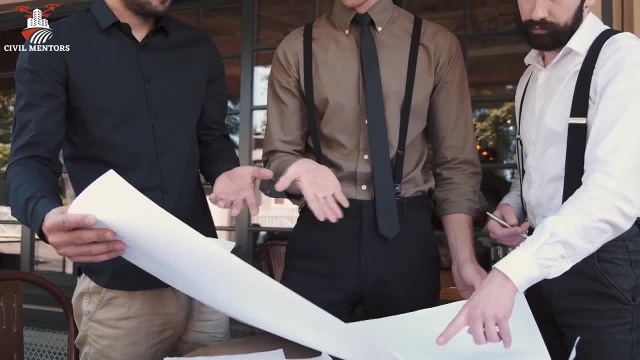 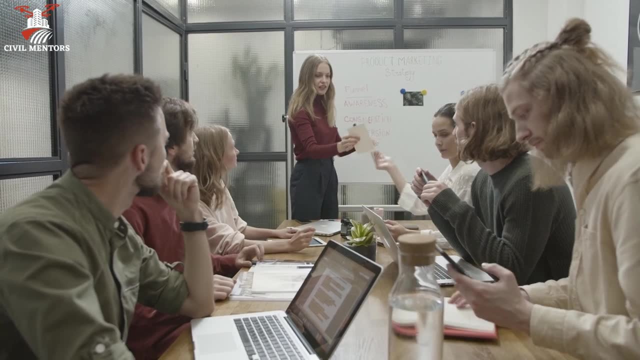 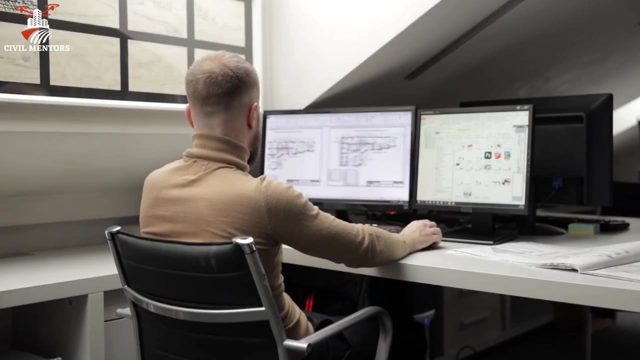 they must be able to convey complex ideas and concepts to clients, colleagues and stakeholders in a clear and concise manner. they also need to work collaboratively with other professionals, such as architects, planners and contractors, to ensure the successful completion of projects. in addition to written and verbal communication, civil engineers must be proficient in technical drawing and 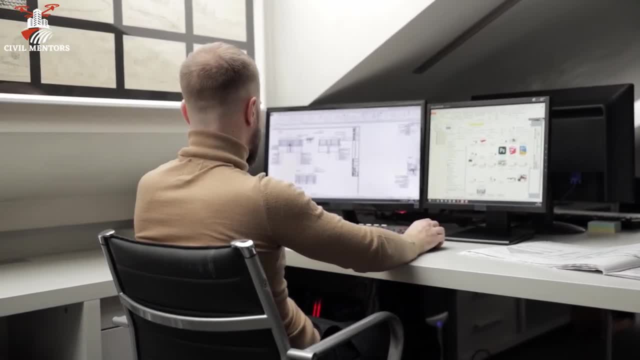 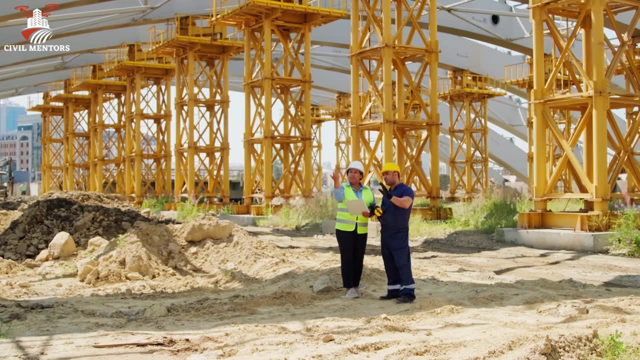 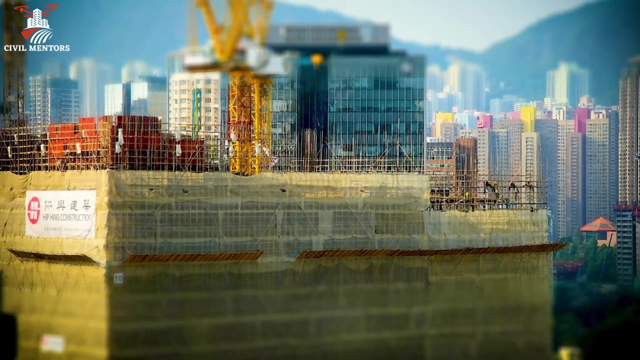 computer-aided design software to create and interpret design plans and specifications. furthermore, project management skills, such as organization management and decision making, are crucial for overseeing projects from start to finish. in conclusion, civil engineering is a fascinating and diverse field that plays a critical role in shaping the world around us by mastering the essentials, such 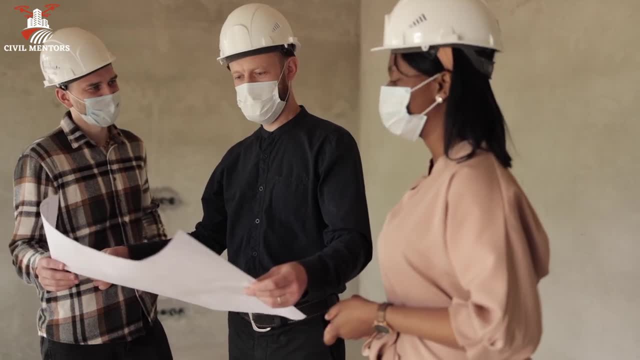 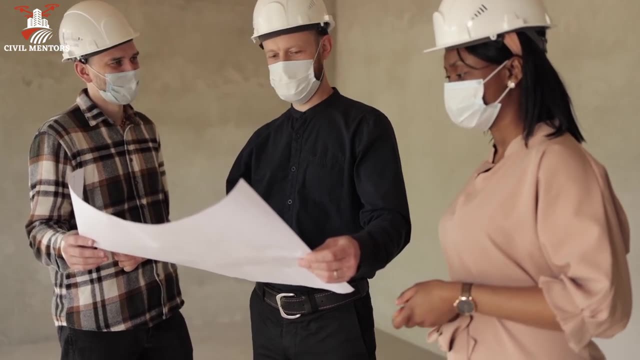 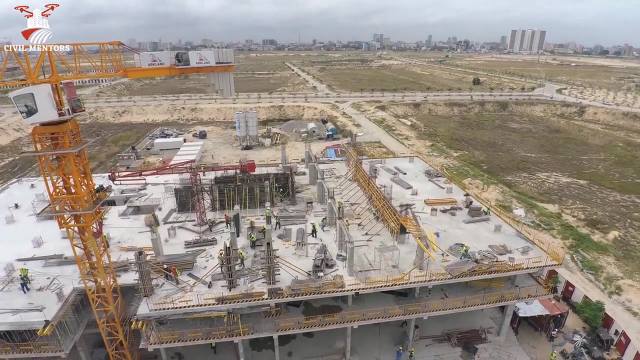 as the key disciplines, design process, sustainable practices, and communication and teamwork skills. you will be well equipped to tackle the challenges and opportunities that come your way as a civil engineer. as you continue to explore this fascinating field, remember that learning never stops. stay curious, keep updating your knowledge and always be open to new ideas and innovations.